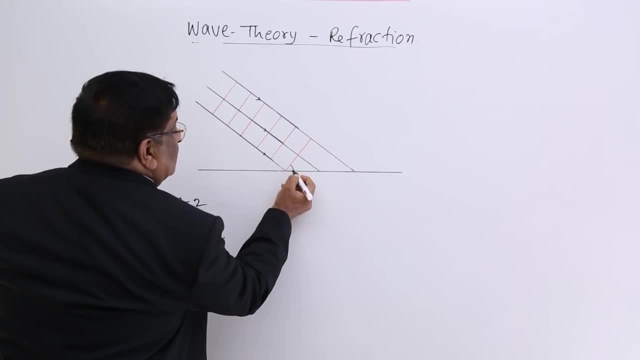 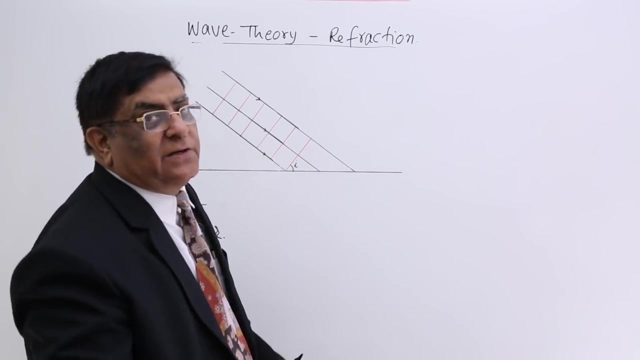 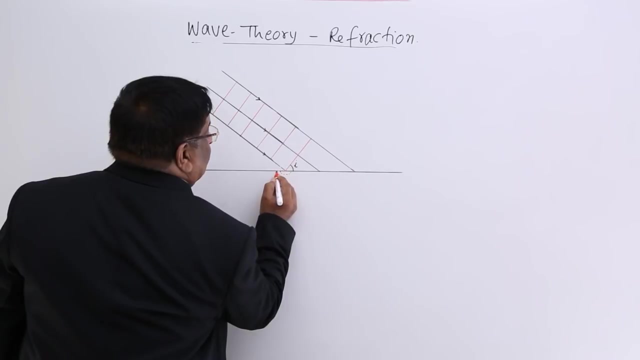 it reaches this point. we say this angle is angle of incidence i, because the two surfaces make angle i. Now all the points of this surface become secondary source. When they become secondary source, they start making their own wavelets. So it start making its own wavelets like this: 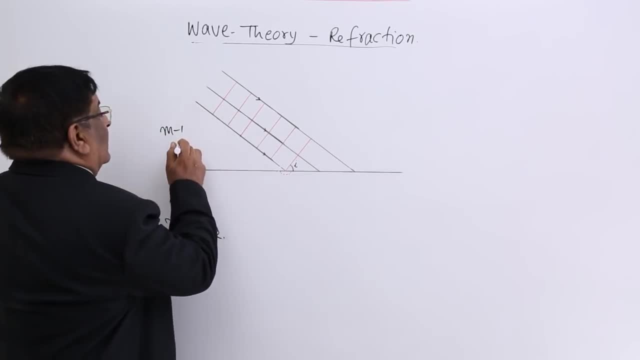 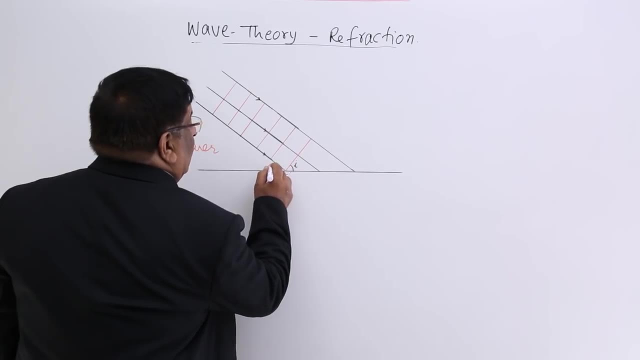 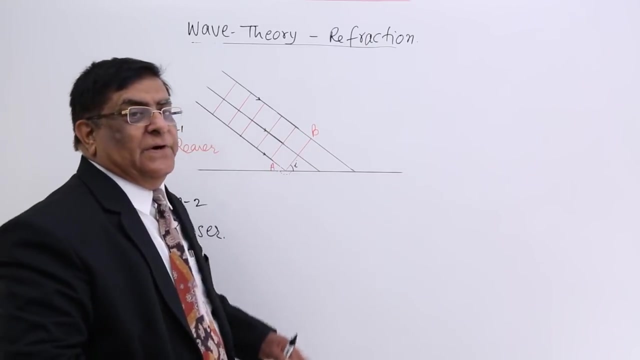 Now this is medium 1, which is a rarer medium, and this is a denser medium. This is A and this point is A. So this is A and this point is A. Now this is A and this point is A. So this is B. A and B. both are on the same front. They start making secondary sources together. 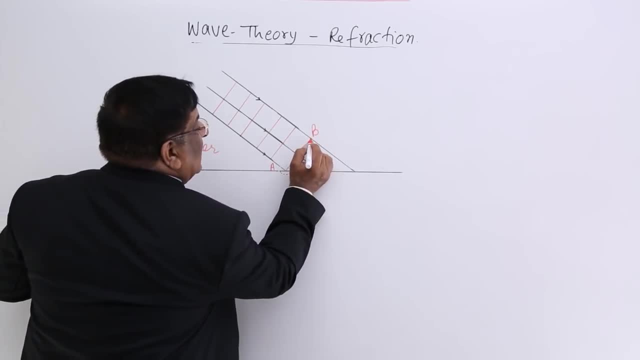 B is making the secondary source and in one second its disturbance reaches here. In two second it reaches here, But its disturbance in this medium, which is denser, in one second it does not reach this much. Why? Because this is a denser medium. 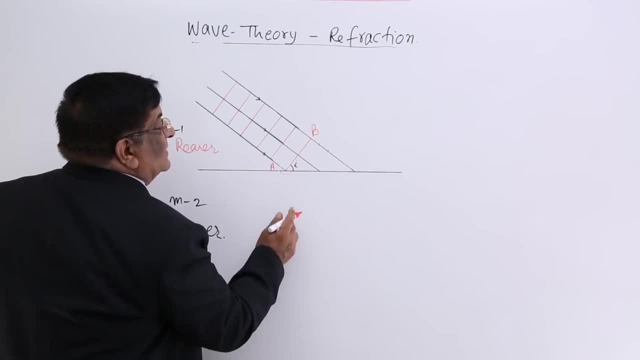 So this is a denser medium. So in denser medium its speed is less. So if the speed is less, it can reach only up to this much. Then in second second it reaches here. In third second it reaches here, You see, every one second. it is taking this much distance, This is taking this much distance. 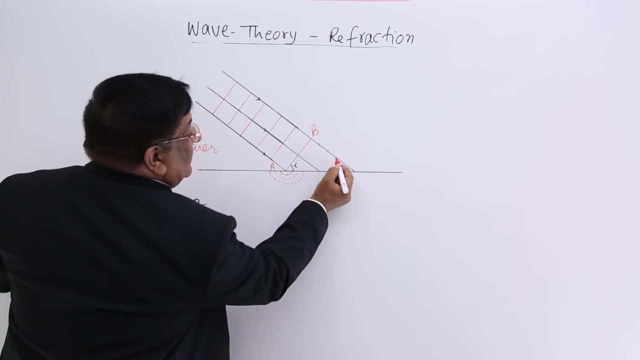 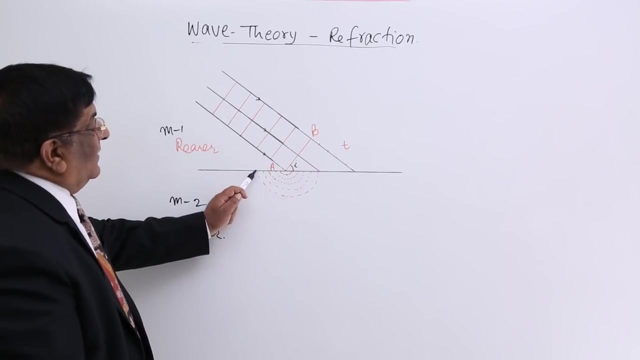 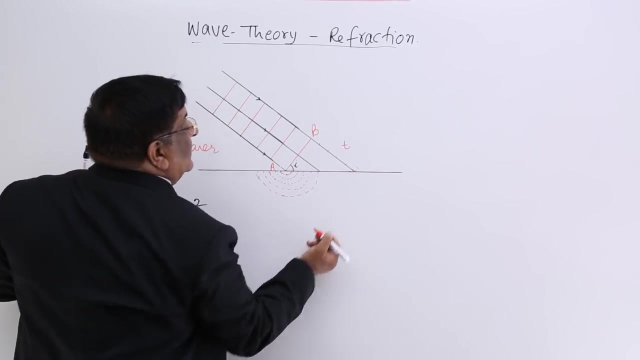 because this is a rarer medium and this is a denser medium. So after time t, it reaches here Time t, And after time t this disturbance is here, The disturbance because of this. point A has made a front here, This B has made a front here. Where is the total wave's wavefront? 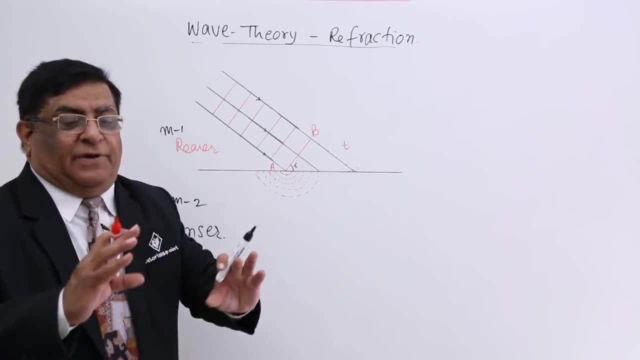 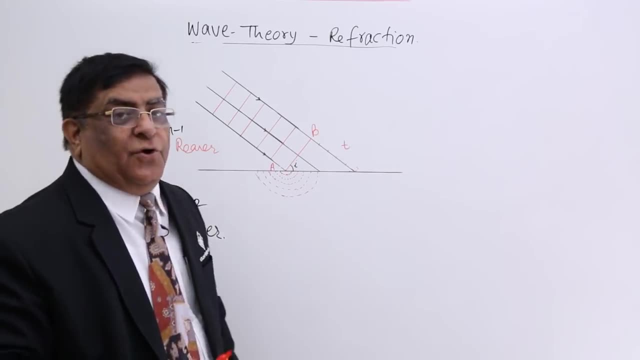 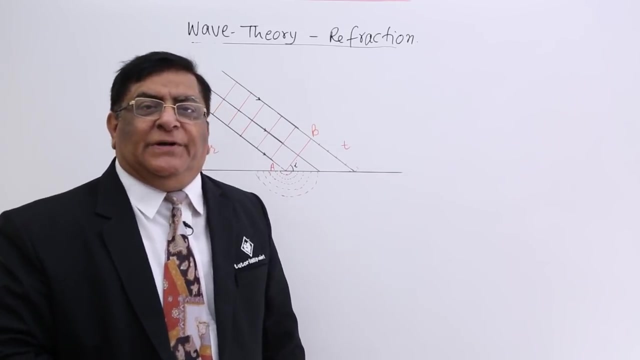 Answer: We have to draw a tangent to all the wavelengths. So if this disturbance is here, this disturbance here, How do we draw a common tangent? In class 10th you have studied how to draw a common tangent. The property of the common tangent is that it makes a right angle with 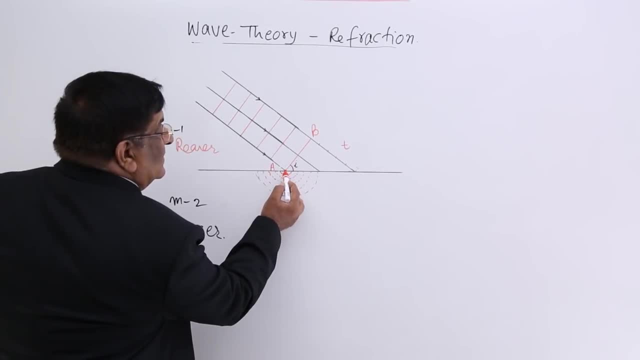 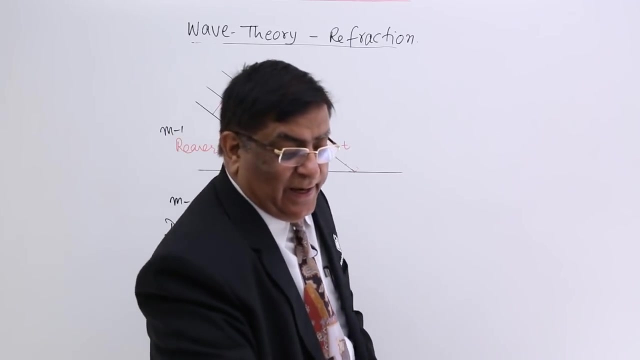 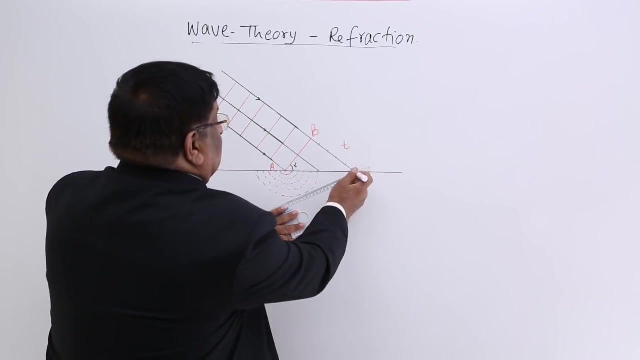 the radius, So all these circles. this is centre. So if there is a radius here, the tangent should be at right angle And that should also be tangent to it. Now, to make it this way, I make trial and error and I find that this, Yes, This is the common tangent. See this, This is tangent to both. 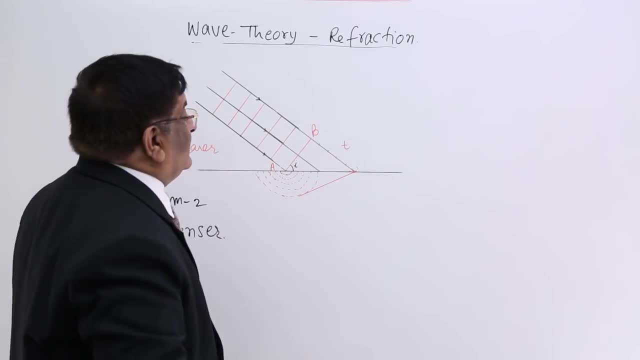 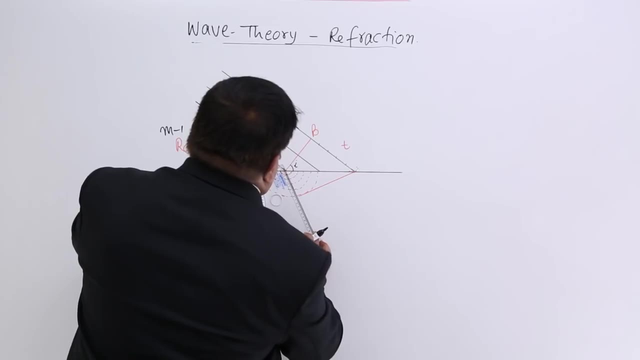 If this is the tangent, what is the direction? Answer: C is tangent to both. So this is the tangent. If this is the tangent of 483.. Let us draw a curve here. See this perpendicular to the wavefront is the direction. This is right angle. This is the direction of propagation. 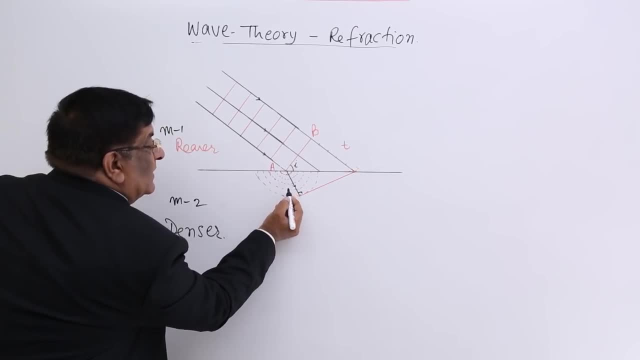 The direction of propagation is always right angle to the new front. This is the new front. How much time has taken from this point to this point? t and how much time it has taken from this point To t� question? The solution is this: t and t is the tangent from current. 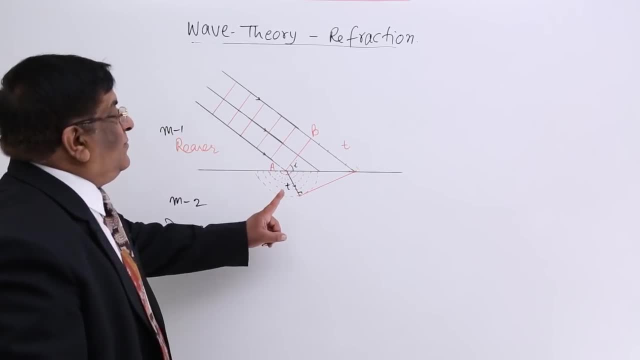 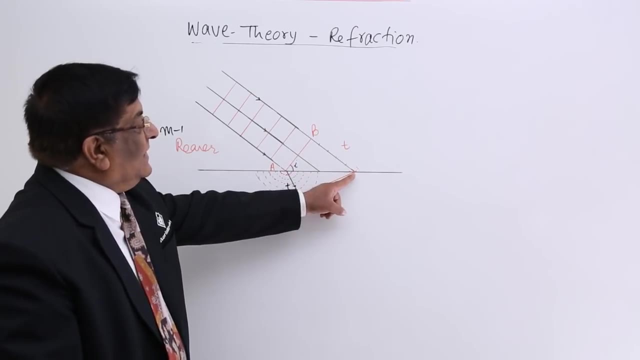 This? no isuelle, Where does this go? i no, This is thesweisell. probably this area is the direction t. So at t point, see this wave front, at t point this has the disturbance reaching. here It is a larger distance because this is a rarer medium. This disturbance reached only 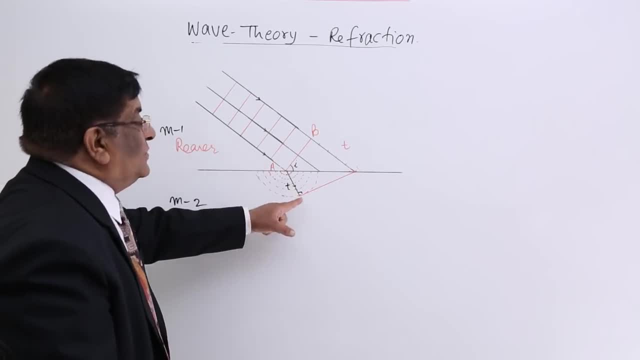 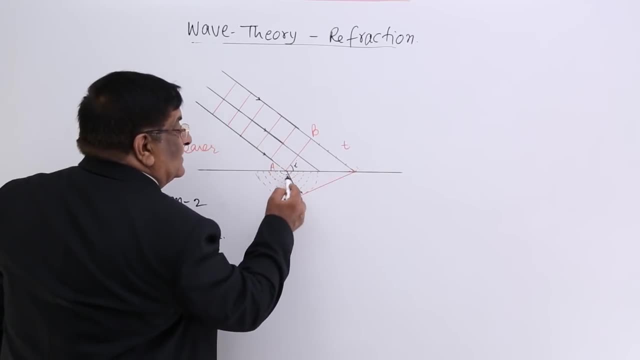 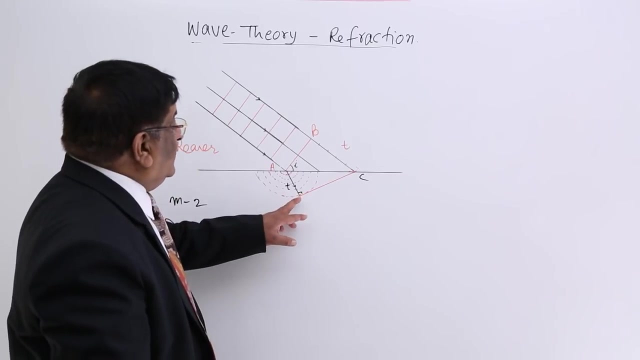 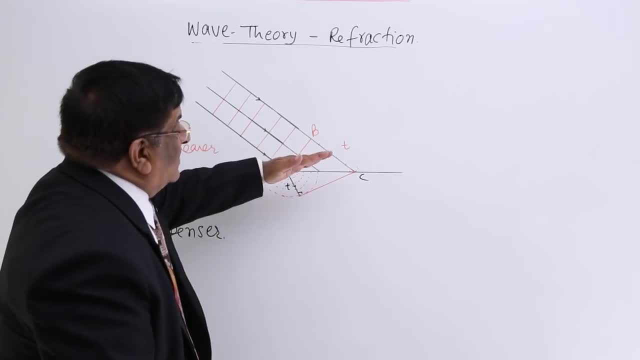 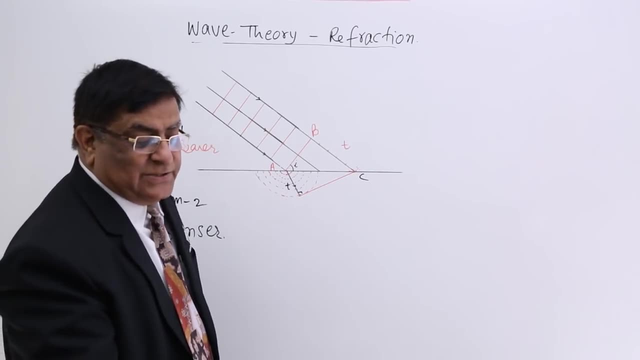 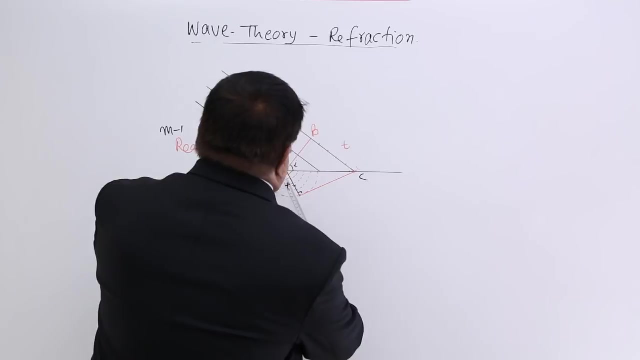 all are in the same medium. Now their disturbances will move at the same pace. and in which direction? Answer: direction of the wave front is always normal to the wave front. So they keep on moving in this direction. So this is the direction they keep on moving and parallel. 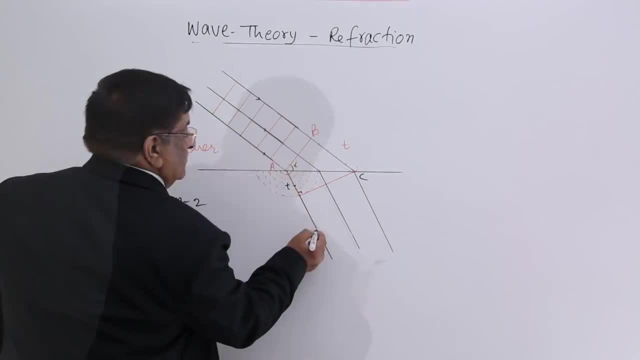 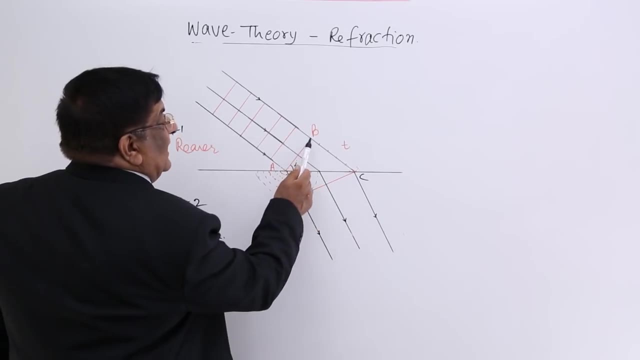 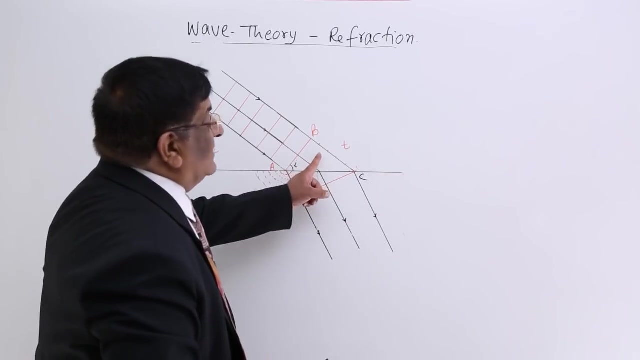 to this and parallel to this, this is the direction of propagation, because this is at right angle. So at time t, it is here, at time t, it is here at time t, it is here. Here: the velocity in the medium y: 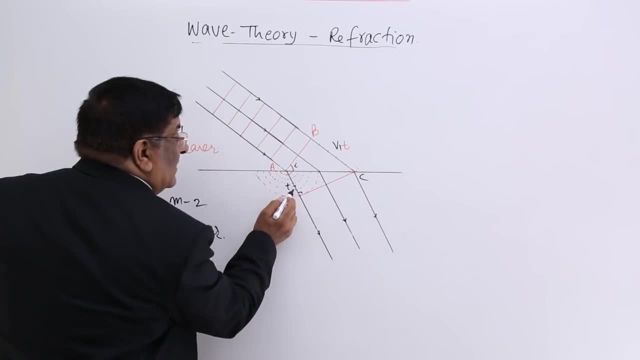 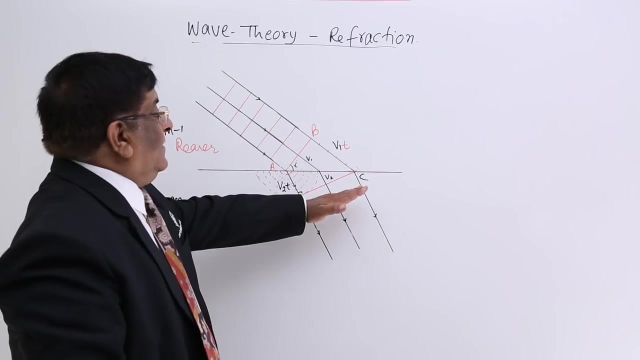 V1 is V1.. Velocity in the medium 2 is V2.. Here V1, here it is V2, and part of the time at both the places. So this whole disturbance of all the points have reached this point. So this is the scenario. Then, after a moment. now it is in the same medium, this wave front. 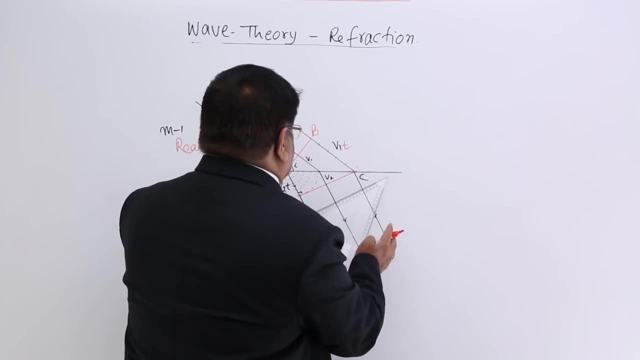 keeps on moving, So V1 keeps on moving. So if the wave in the medium 2, V2, V3,, V2,, V3, V2 and so on, Then V1 keeps on moving in forward direction, like this: 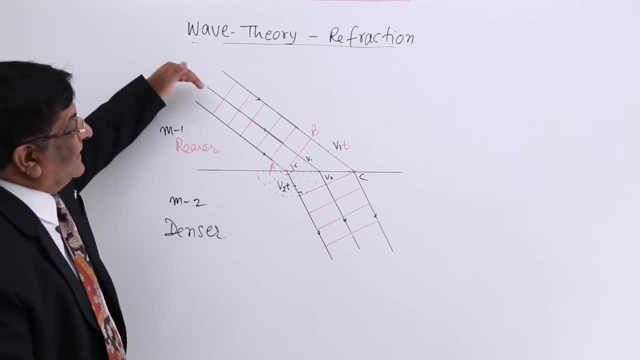 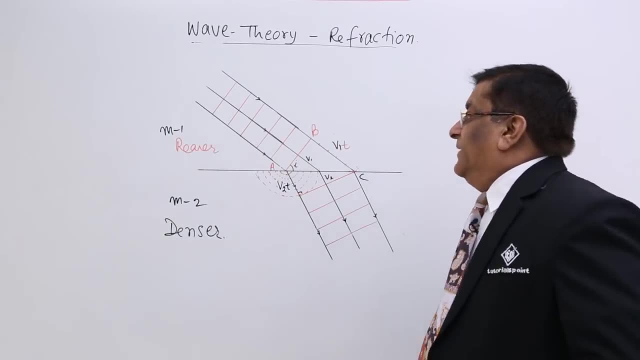 This way it keeps on moving. So you are seeing something. I am also seeing the same thing. The direction has changed. This is what happens in. we can explain by the wave. In the second medium the speed of the wave is less than V1.. So here V1 is V2, V3, V3, V4 and V4, and 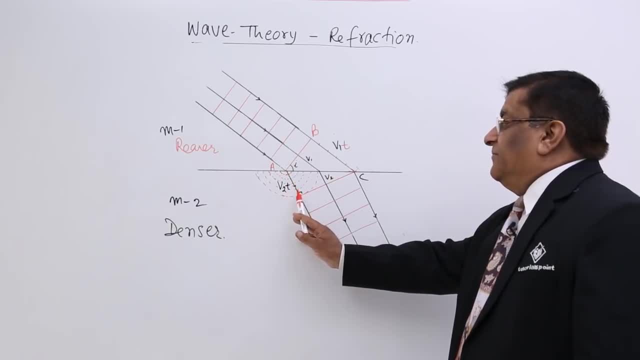 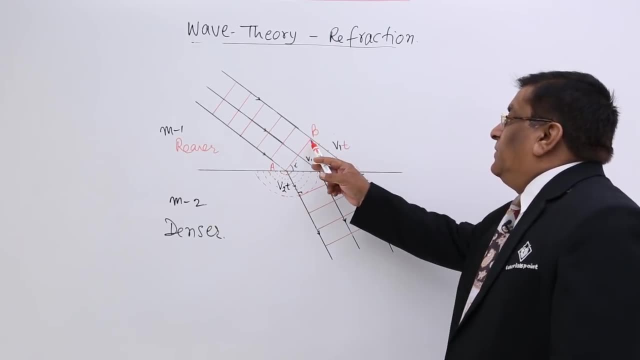 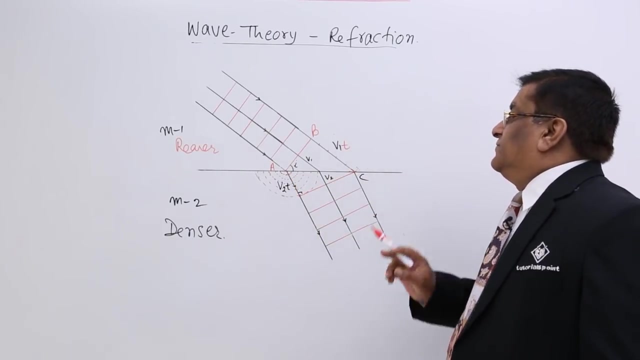 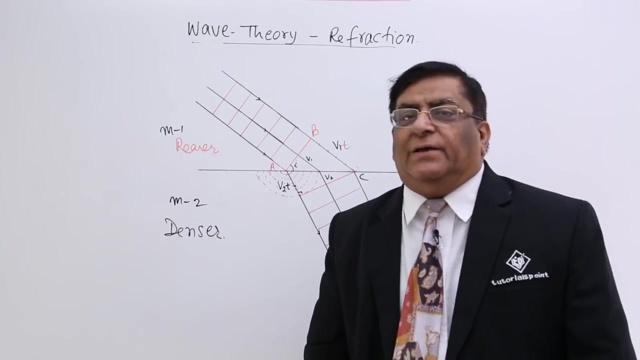 the wave is less and this disturbance is in the wave. Here it is still in the first medium. So this is fast, this is large, this is small, This is V2,, this is V1 and this is the reason that there is a bend in the direction. So if somebody asks why the light direction changes, 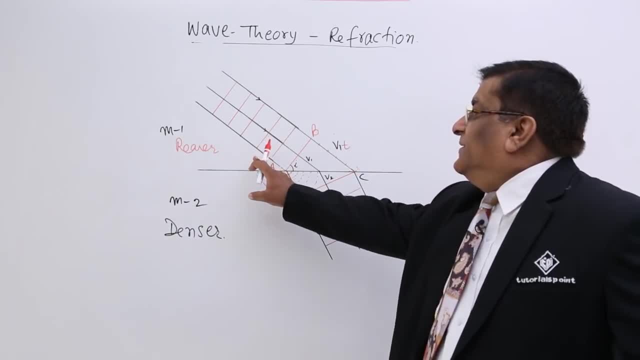 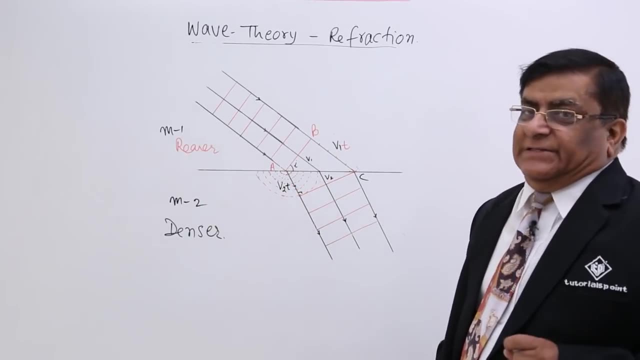 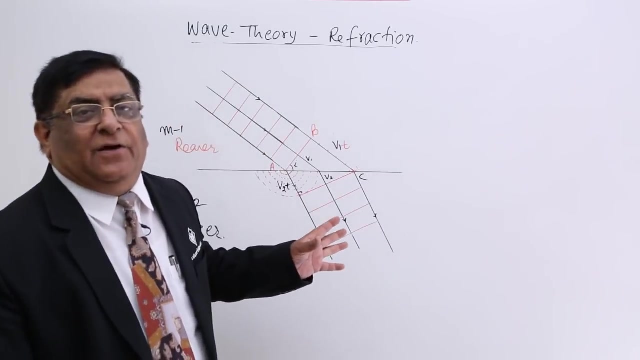 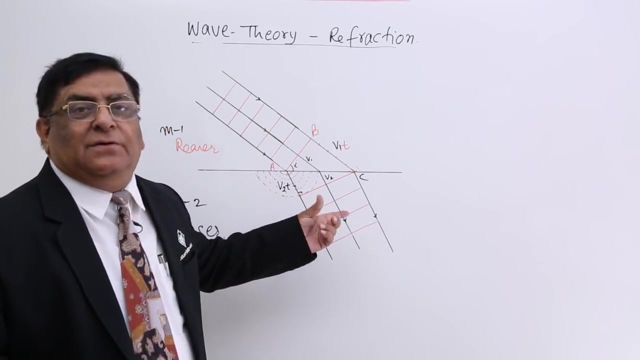 why the light direction deviate in the denser medium? Answer: because velocity in the two mediums are different. This is the reason. Now we have explained why it bends by the method of waves. Now we have to find whether law of refraction are having good here or 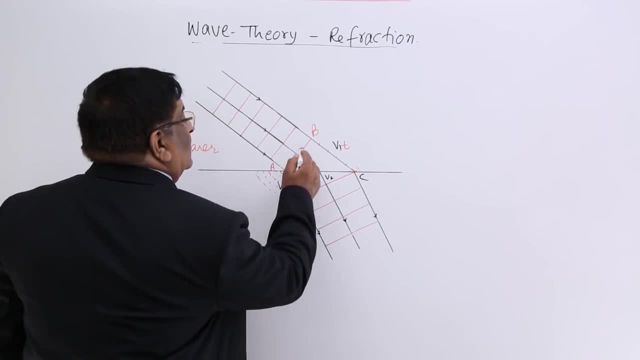 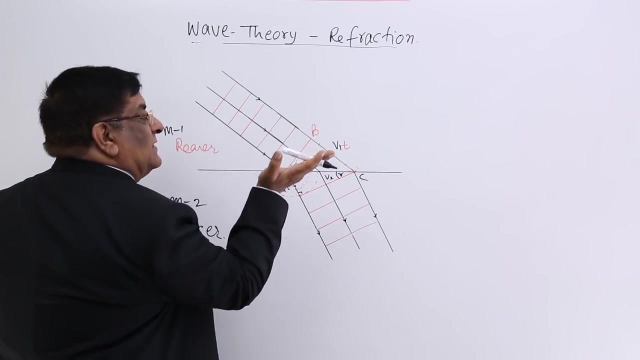 applicable here. This is the last wave front making angle of incidence. This is the first wave front, This is the wave front parallel to this. So direction of this wave front with this surface is R. angle of refraction Wave front and the surface of the liquid or the surface interface. So 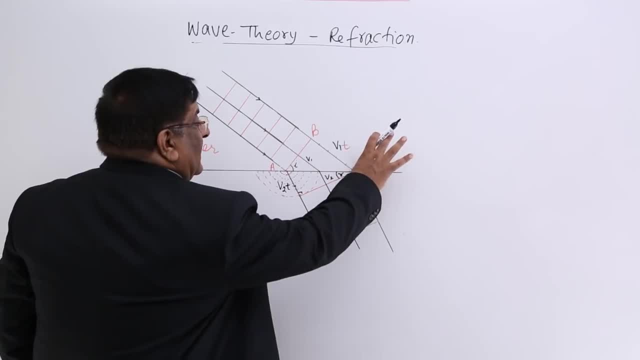 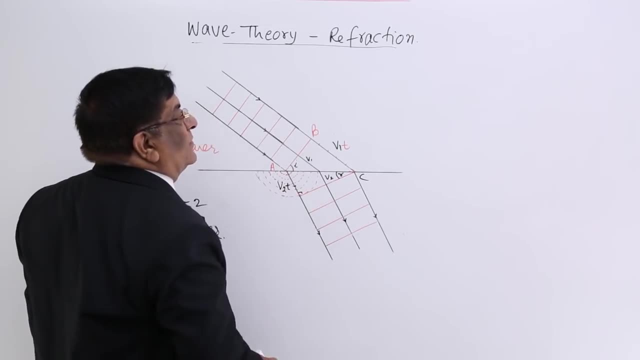 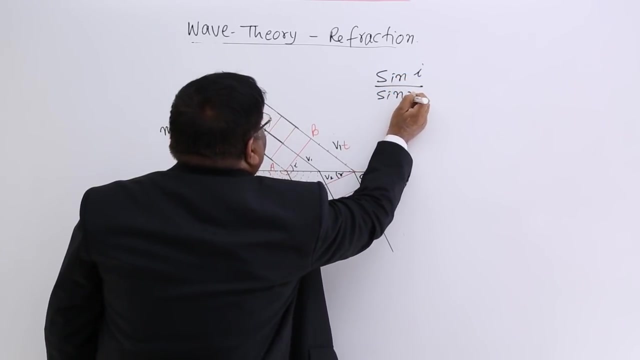 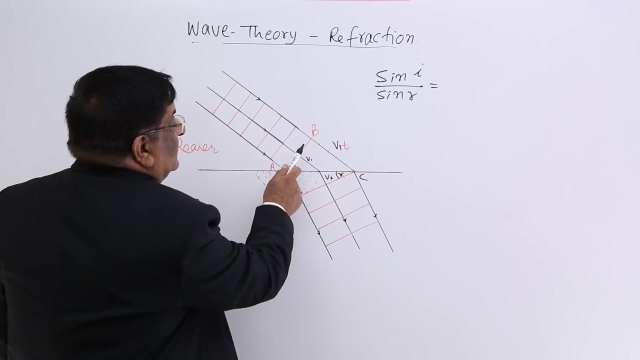 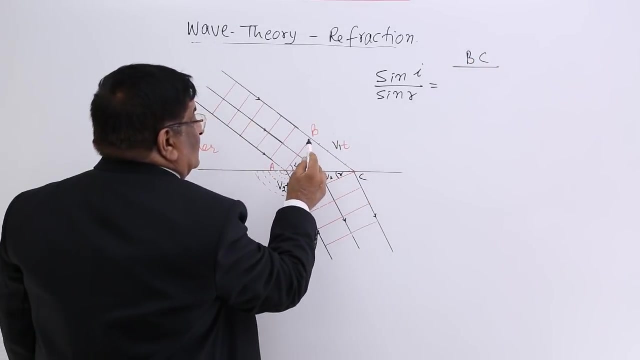 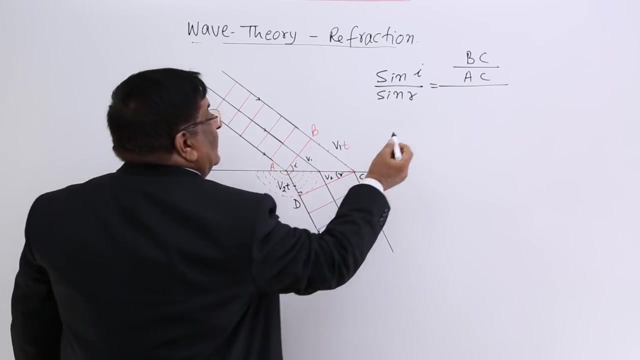 this angle is angle of refraction After refraction. this is the first wave front. Now here sin I upon sin R, sin I perpendicular upon hypotenuse. This is perpendicular BC, hypotenuse AC. This is to be divided by perpendicular A, B, C, D. perpendicular AD: This is to be 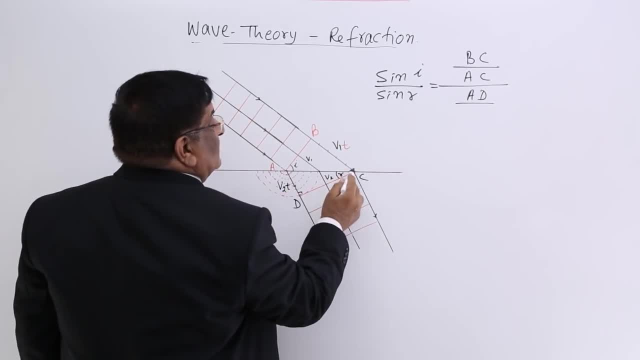 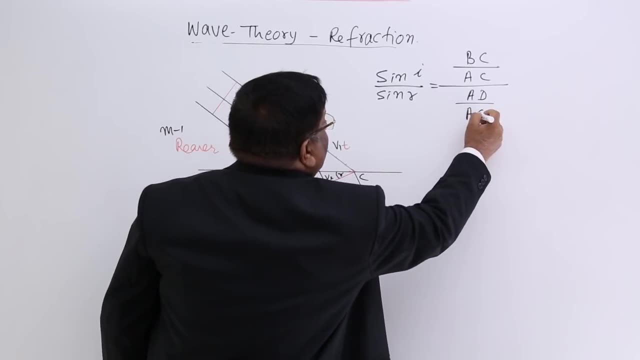 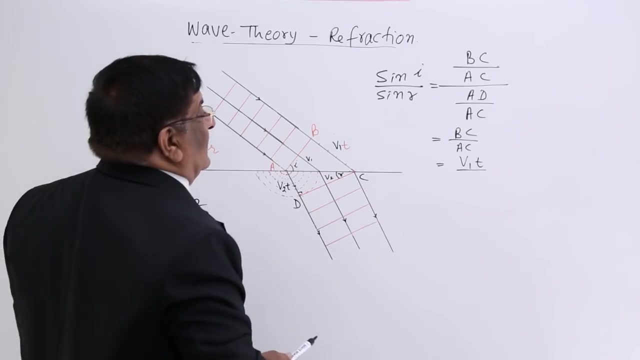 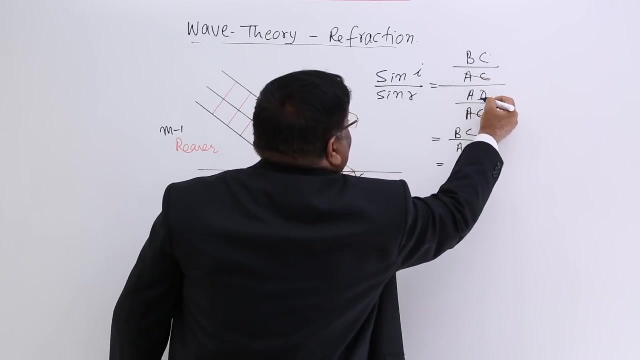 divided by a perpendicular- sorry, hypotenuse AC in this triangle For R. this is perpendicular, this is hypotenuse AD upon AC. Now you see, AC is cancelled, AD upon AC. that is right. AC was cancelled. So what we had here is BC. this is cancelled, BC upon AD, BC upon AD and 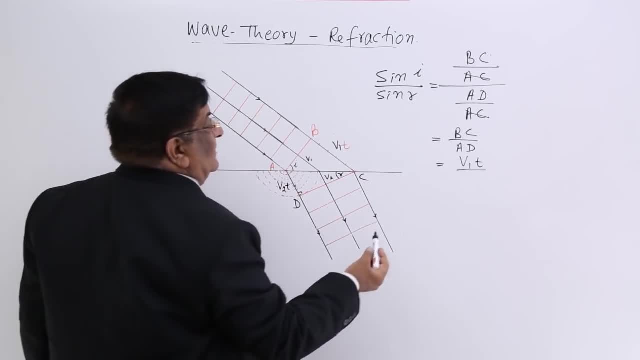 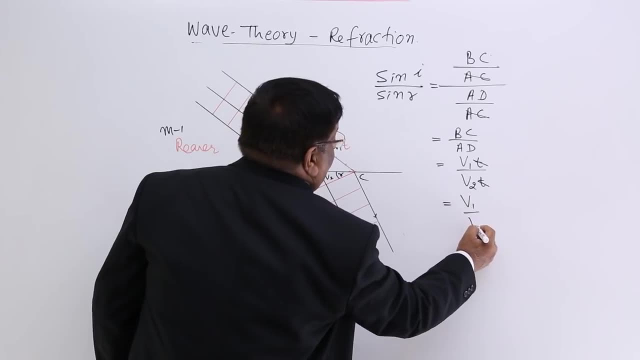 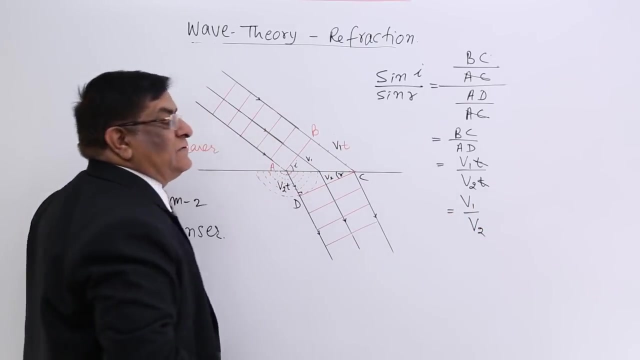 this AD is equal to V2 into T, V2 into T. Here T is cancelled and this AD is equal to V2, and what we get is V1 upon V2.. This is velocity of light in medium 1 and velocity of light in medium 2.. Now for velocity. 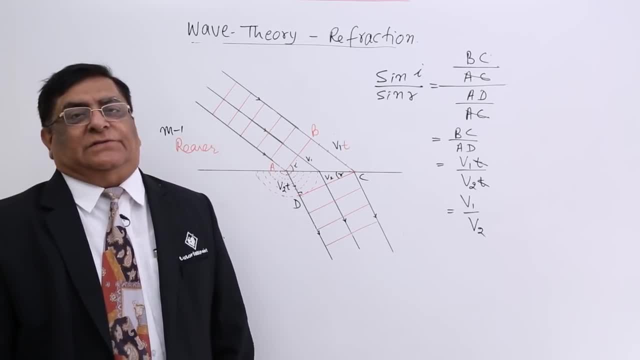 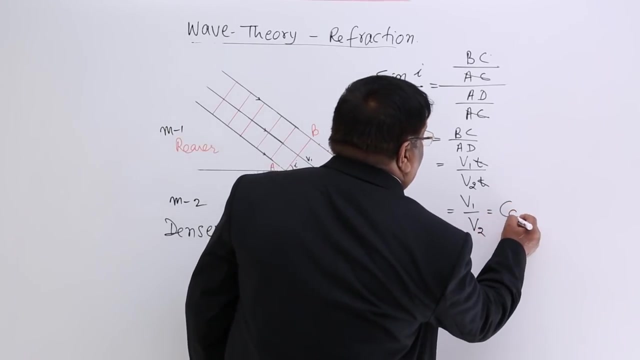 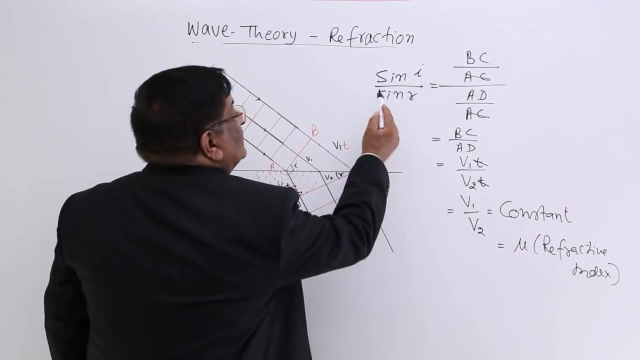 of light in any medium. it is a constant. Velocity of light in a single medium is constant. it will not change unless medium is changed. So here, V1 is a constant, V2 is a constant. So this is also constant. And we know the name of this constant is mu refractive index. What is this? sin i upon? 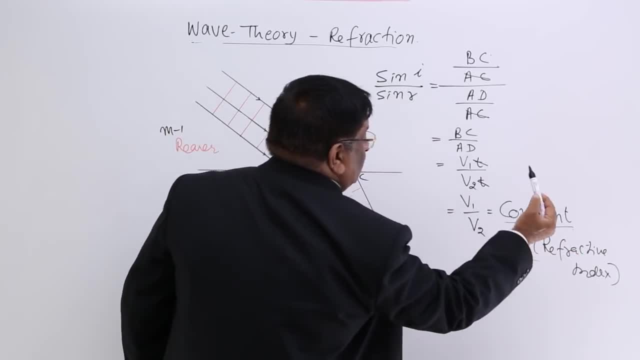 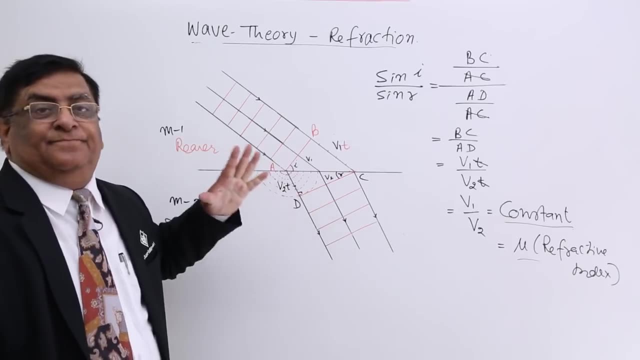 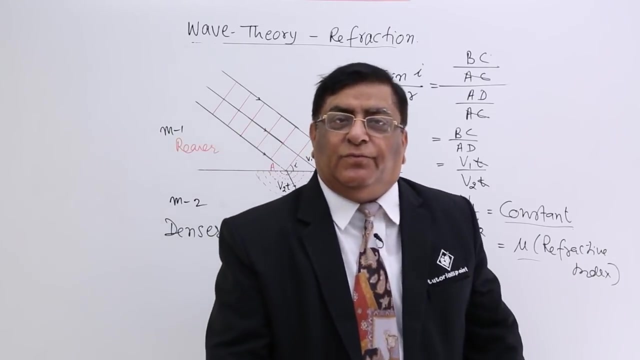 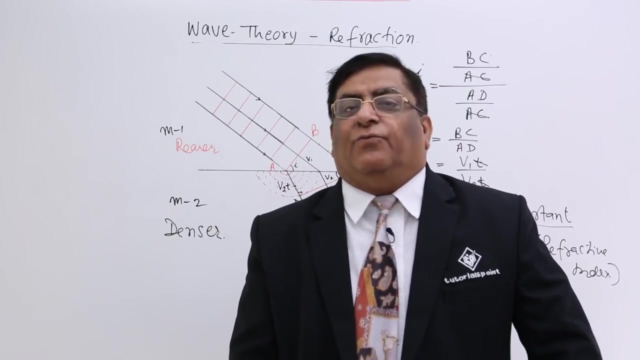 sin r is constant and that constant is refractive index. This we have proved by wave theory. So this is wave theory. we have proved refraction. So in this way we proved reflection and refraction. And we also know that by Newton's effect we can. 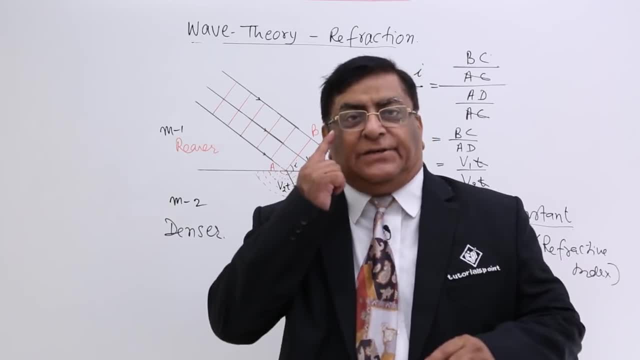 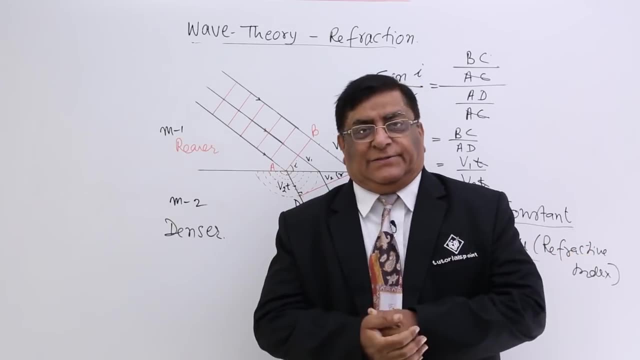 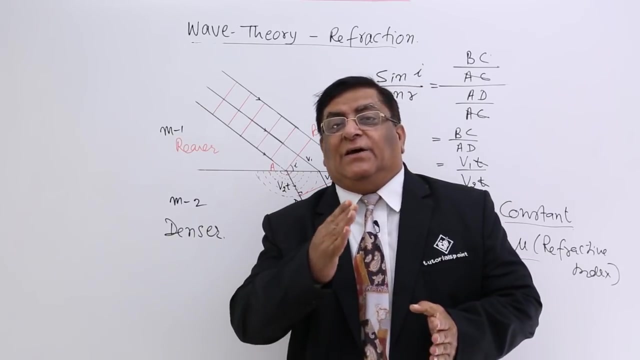 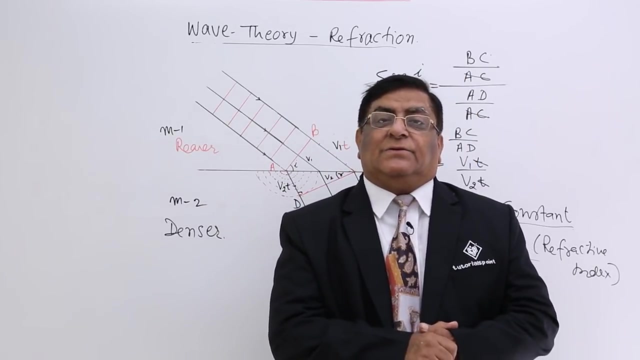 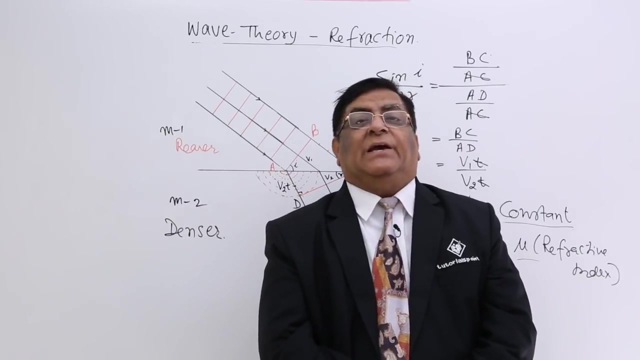 solve any coated current with field. So in this way we can solve any coated current with field. Then we 되게 the feature of optical ray, Eye ray, Energy and profits of the pay. us know low probability growth. So Huygens, he thought about this, that if there are waves then there will be a phenomena. 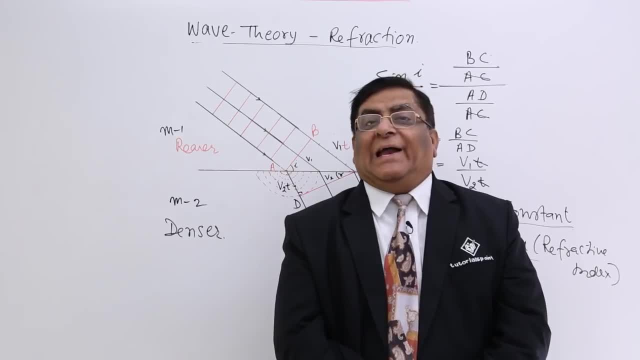 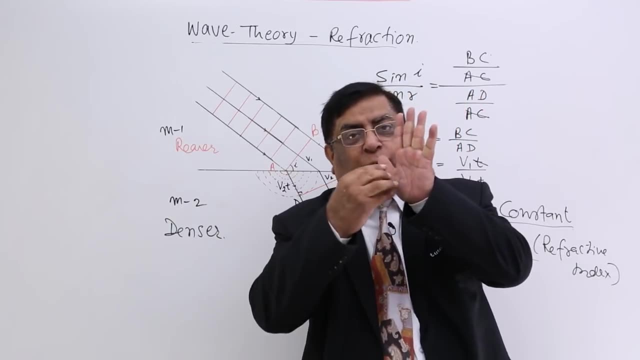 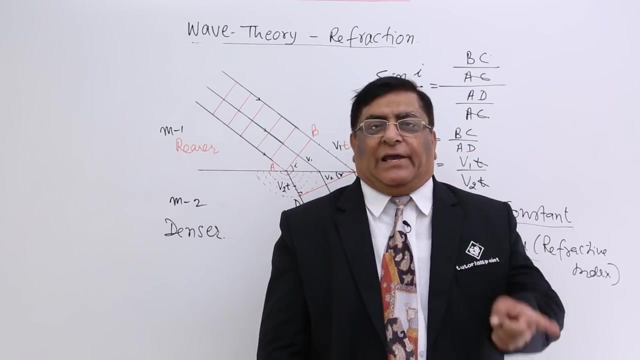 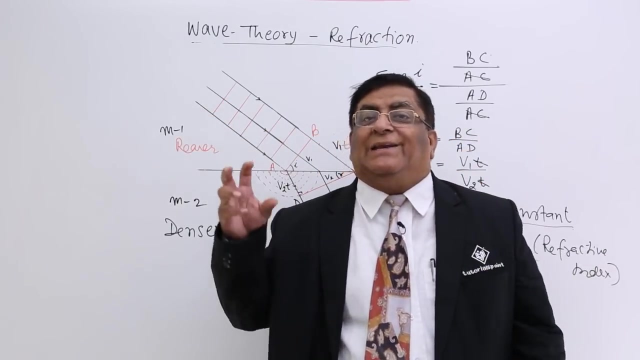 of superposition of waves. and with the help of superposition of waves we will be able to make certain spots where the intensity of the light will get added up again. If there are two sources of light, then the light by one source can cancel out the light. 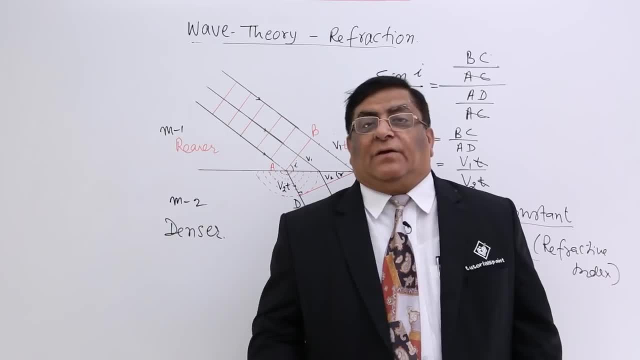 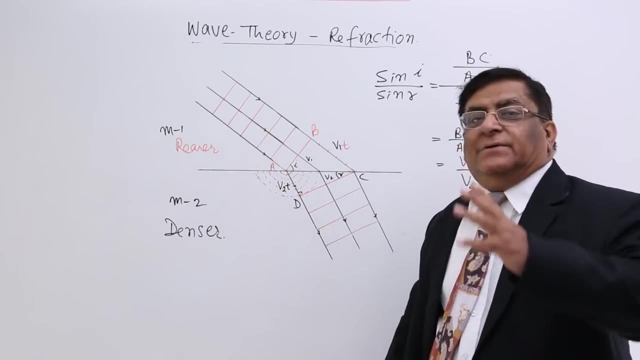 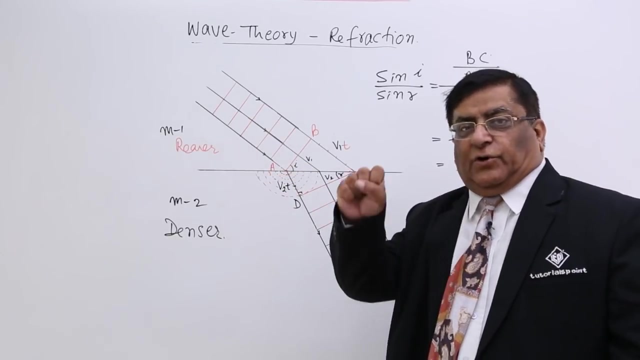 by the other source. Again, one source is giving light to this wall intensity: I switch it off. Other source giving light intensity: I switch it off. Start both the sources. How much is intensity? 2 I, 2 I, ok. 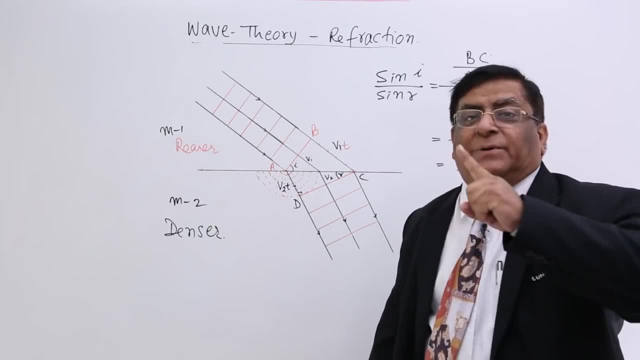 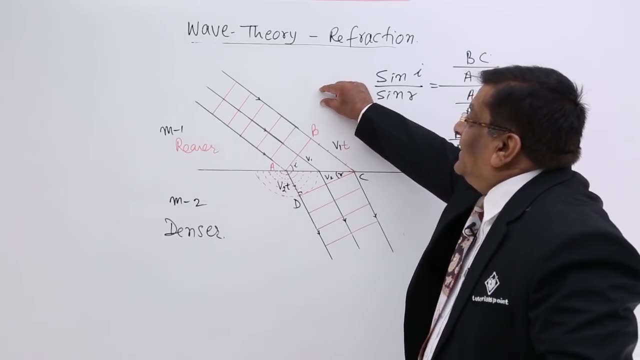 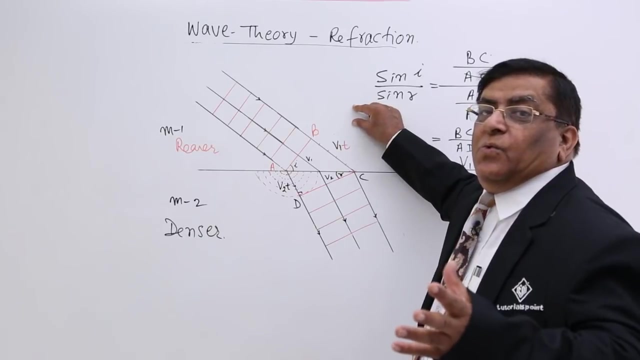 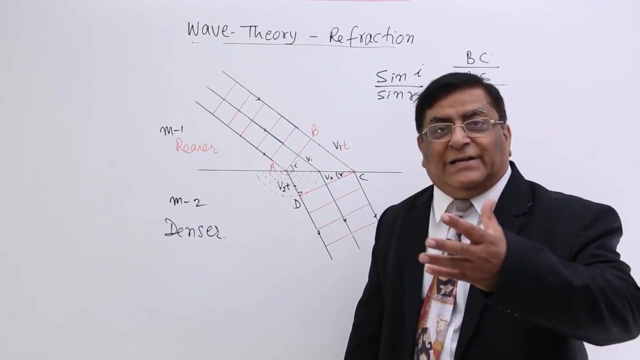 Then he said that there can be. there can be a situation when I will see the intensity of light equal to 4 I, and here intensity is 0.. Intensity 4 I. intensity 0. Zero intensity means what Darkness? and there are two bulbs. 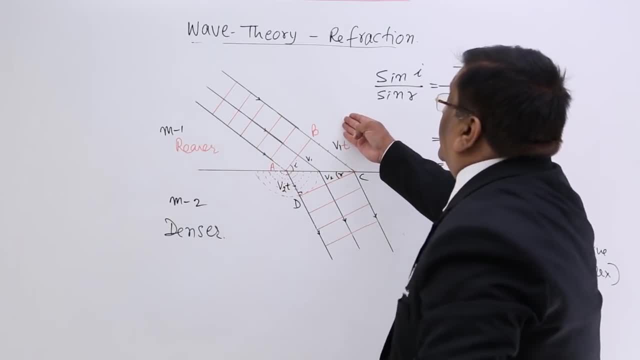 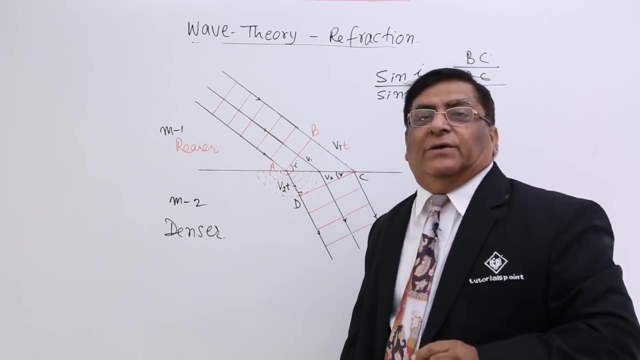 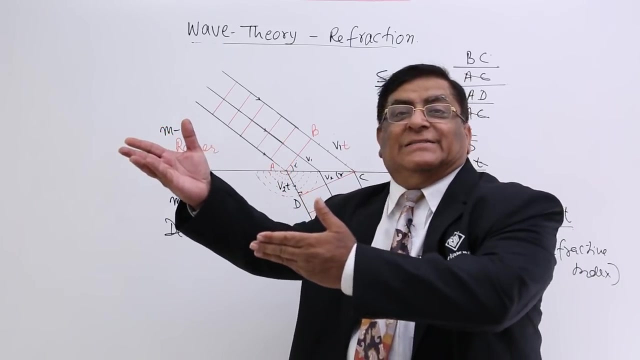 If there are two sources of light here, how much light you get? Zero, This is possible. That is what he said, and he explained by theory that, how this is possible, that we are having two bulb, two sources of light, and what we are seeing is darkness. and he explained it. 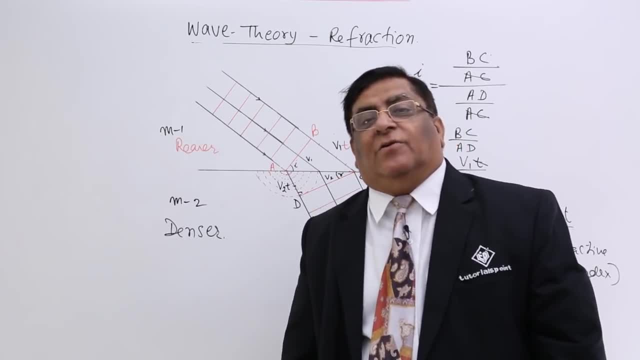 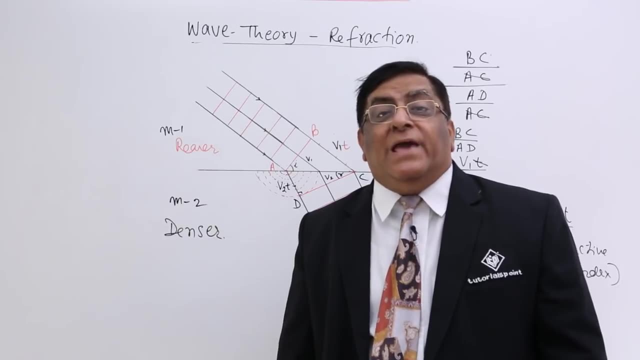 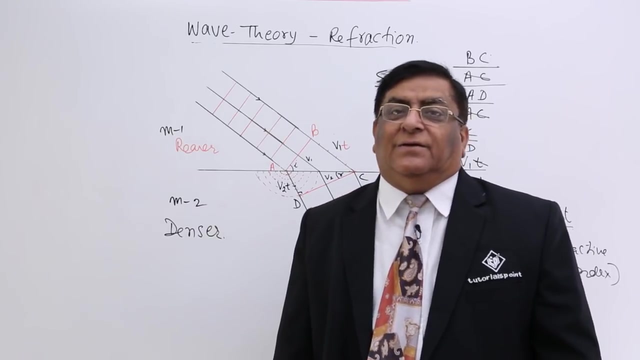 But people did not agree. They say it is good on the paper. You show it by experimentally. Then only we will agree that this may happen. He could not show it, but his student, young, could make it, and he has shown it, and at that.